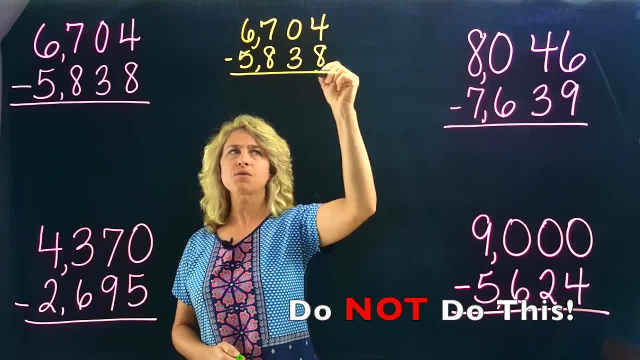 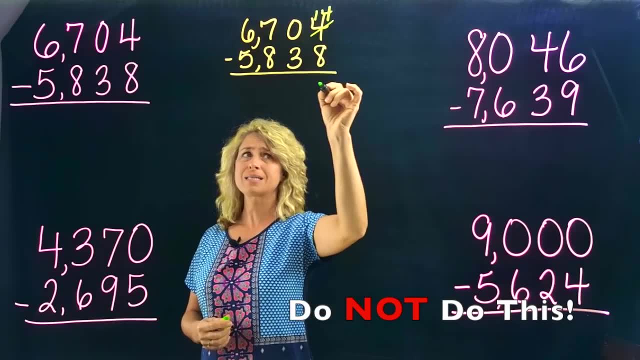 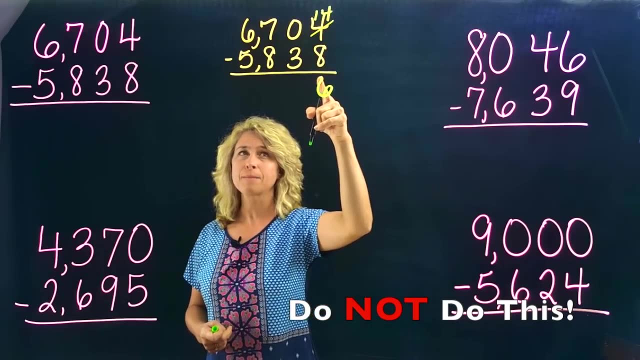 some of my brightest students do this. they'll take this first number and they know they have to regroup, and they make this a 14 to start with, and then they say 14 minus 8 is 6. this is an absolute no-no, and this is why, if you do that, you 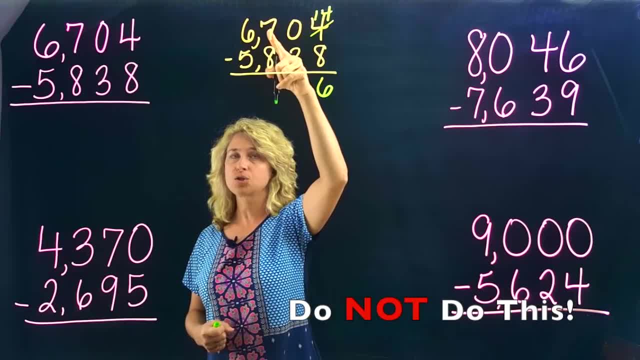 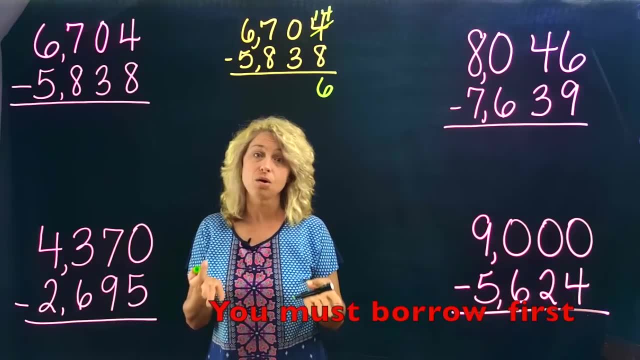 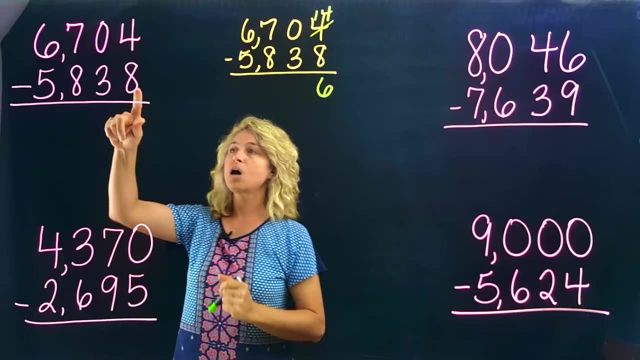 may forget that you need to borrow next door. so always borrow before you can spend. it's like going to the store: you can't spend money you don't have, so borrow before you can spend. borrow first and then spend it. watch this, so here's what to do. you know you. 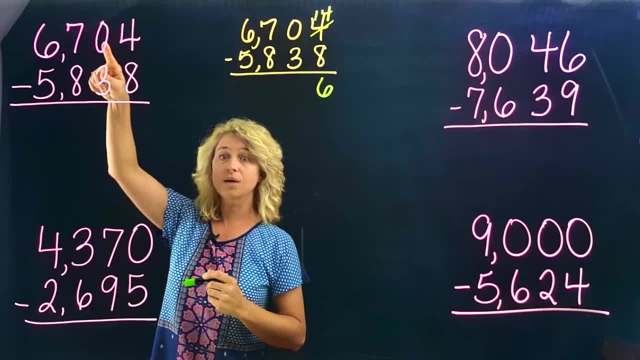 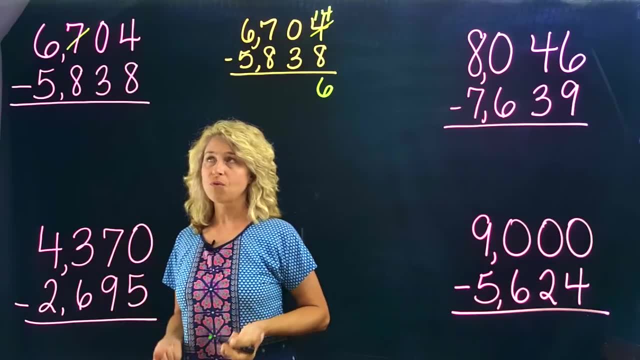 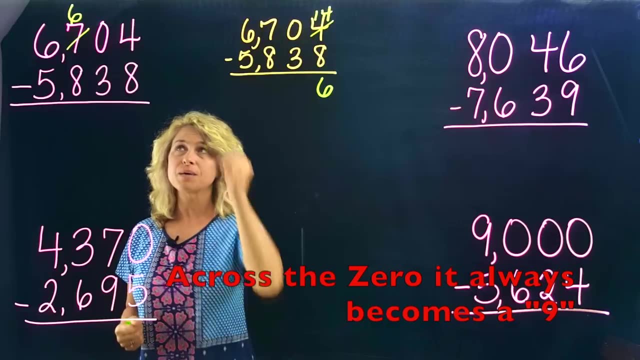 cannot take 8 from 4, so borrow next door. you cannot borrow from a 0. go to the next group over here. borrow 1 from 7 is 6. now, when you're going across a 0, it always becomes a 9. technically, you know it's a 10. 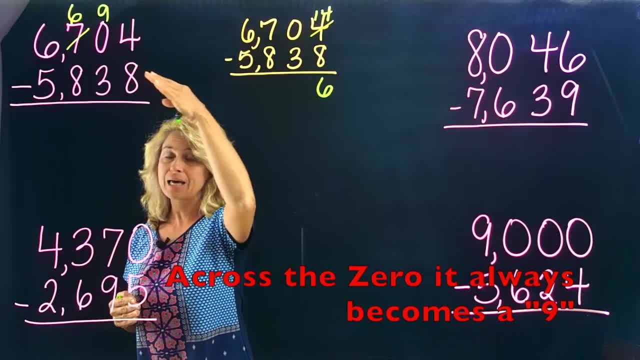 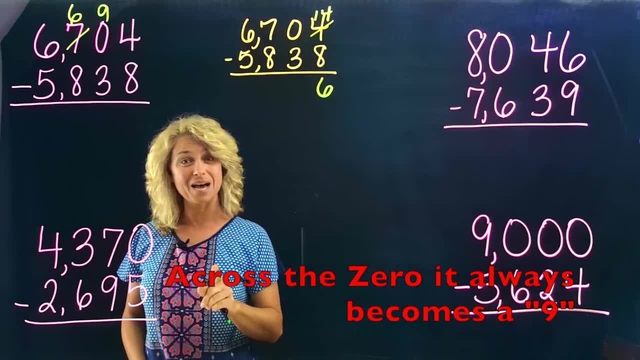 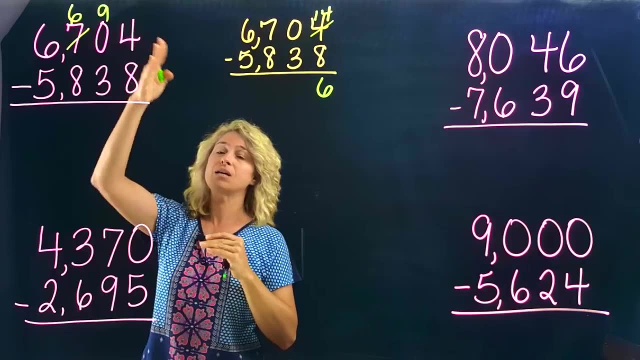 and then you borrow 1 and make it a 9, which is 1 less. but anytime you go across a 0, just make it a 9 and save yourself a step. now we have the 10 that now we can spend the money. we can put the 10 on the 4 and it can become 14. 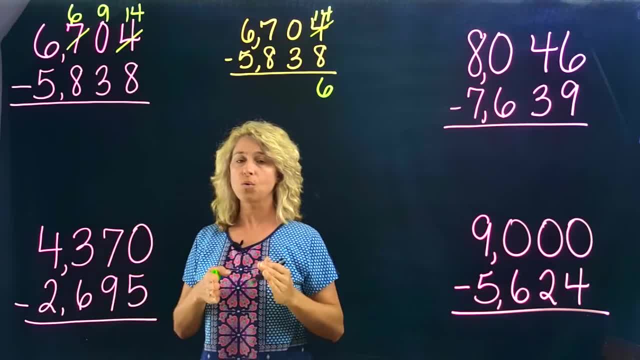 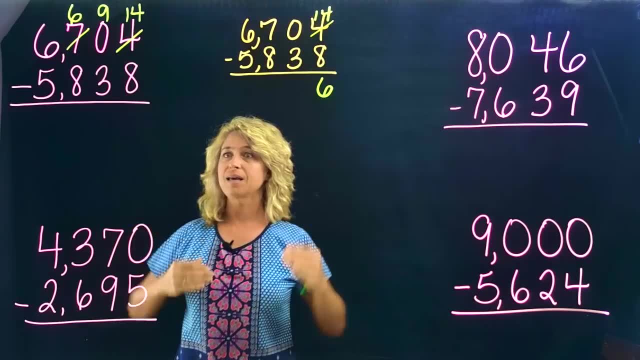 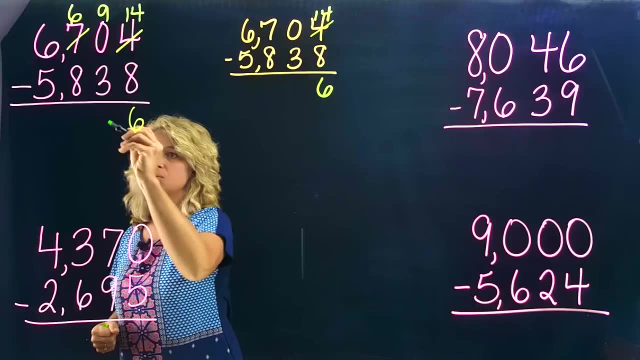 this is the proper way, in the proper order, to be able to regroup. do not do this, you'll forget and you'll be sorry. alright, so here goes: 14-8 is 6, 9-3 is 6. can you take 8 from 6? now we are going. 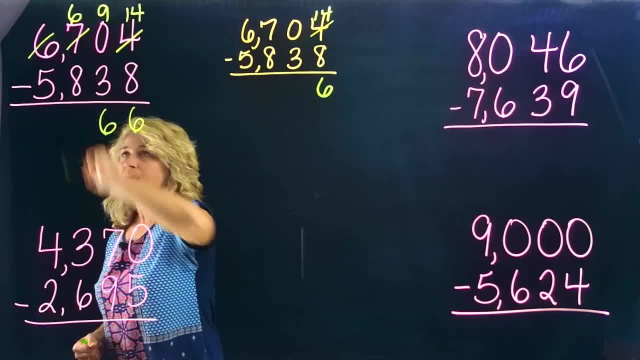 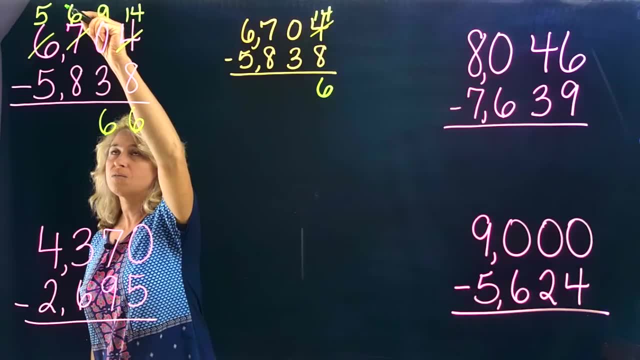 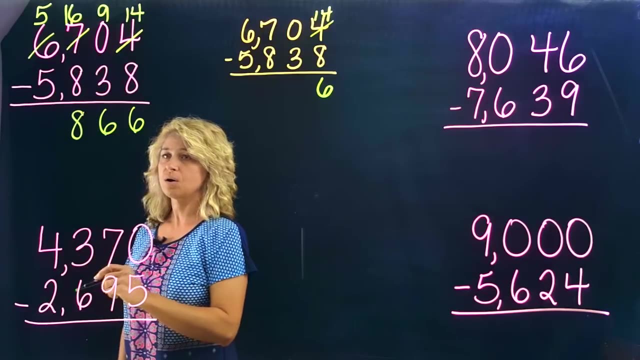 to have to borrow again. do it right here, then 6 forms, 5, more forms, 8 and 6 on this column is 16.. 16-8.. does it is 8, and 5 minus 5 is 0. so our final answer is 866. so you notice. on the first, 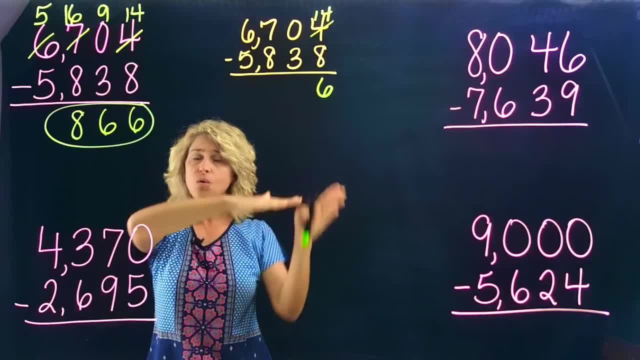 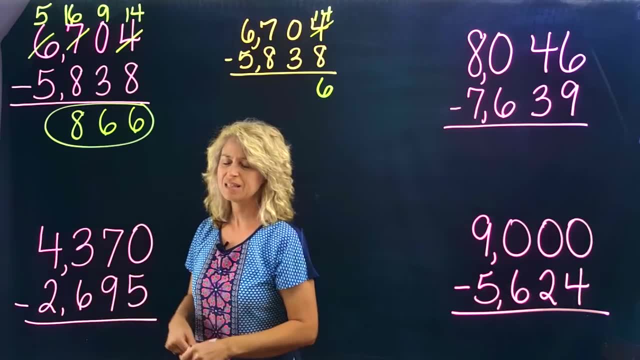 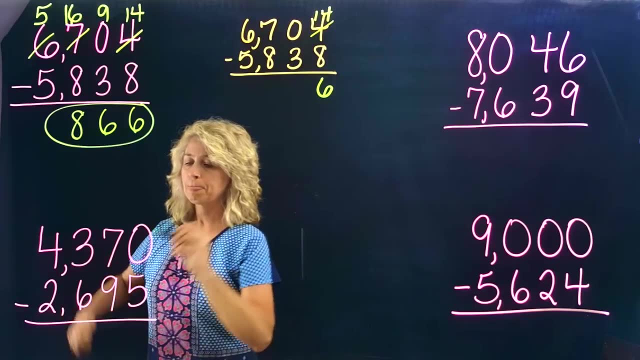 example, the thing to remember is: when you go across a 0, make it a 9. let's look at this example. the 0 is in a different spot. let's see if it makes a difference. we're going to take 5 away from 0. you can't go next door. make it one less, the. 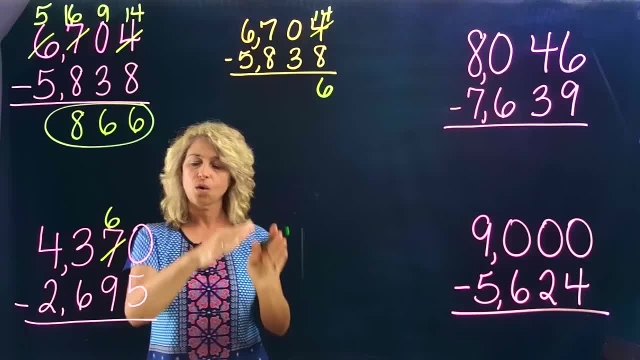 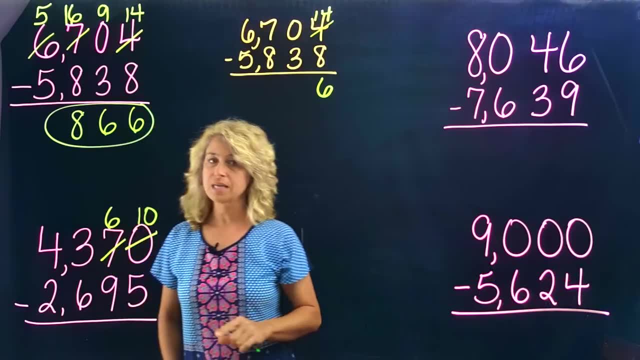 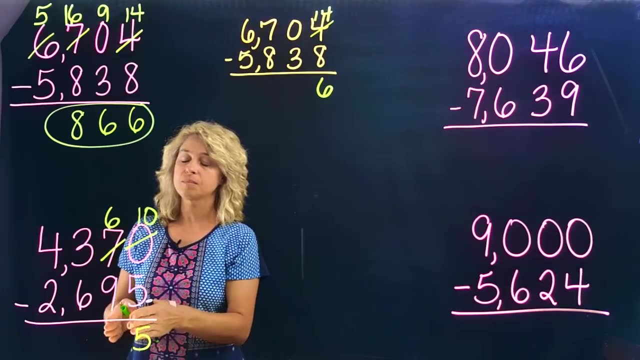 7 becomes 6. oh, we're not going across the 0, we're stopping at 0. when you stop at 0, it becomes a 10 every time. now 10 minus 5 is 5. move on to the next column. can you take 9 from 6? no, you can't borrow next door. this becomes one less. 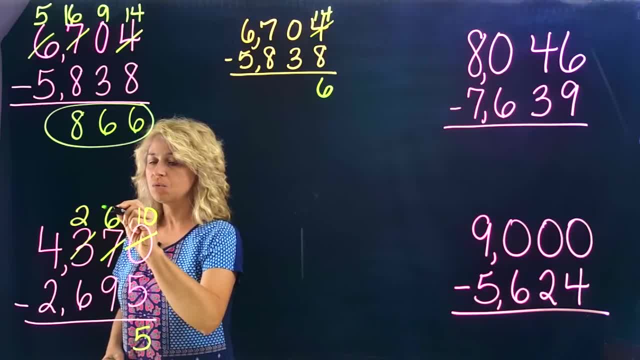 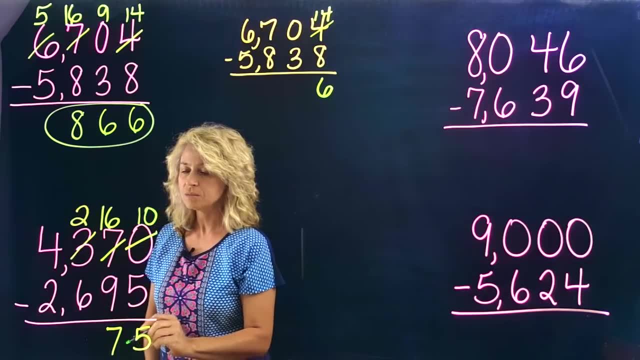 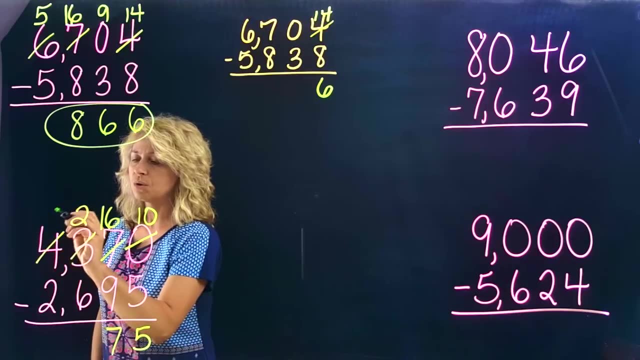 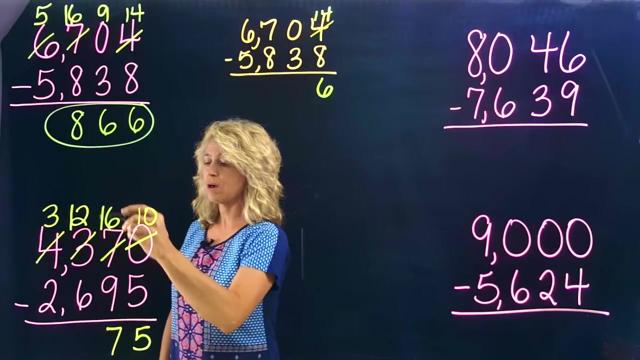 which is a 2. now. add 10 to the one right here. this becomes 6, 16. 16 minus 9 is 7. go to the next column. can you take 6 from 2? no, you cannot borrow next door. make the 4 one less. add your 10 to the 2, which is a 12, now 12. 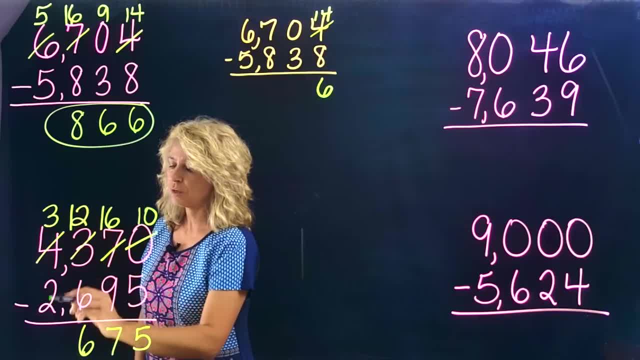 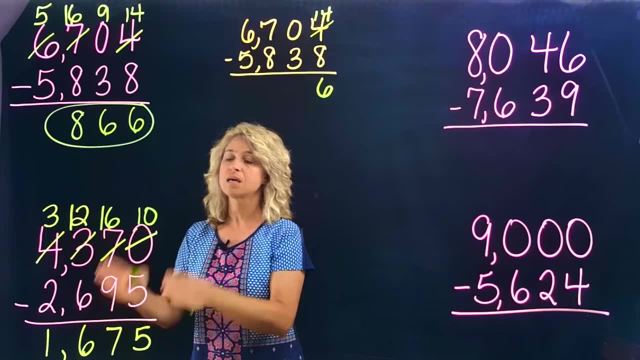 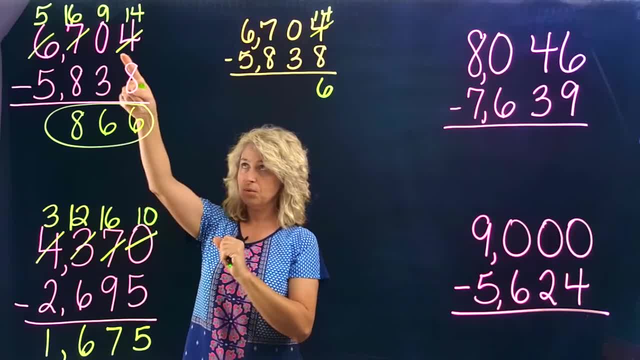 you start a new problem, you start a new problem. you start a new problem. you stop at 0, it becomes a 10. you stop at 0, it becomes a 10. you stop at 0, it becomes a 10. remember here, when you go across, it is a 9. 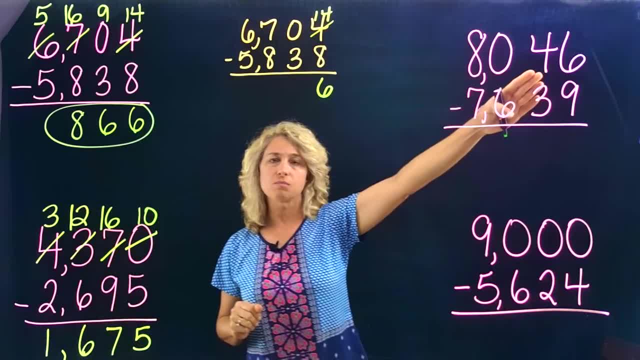 remember here, when you go across, it is a 9. remember here, when you go across, it is a 9. let's look at the next example: the 0 is. let's look at the next example: the 0 is. let's look at the next example: the 0 is moving. the 0 now is in a different spot. 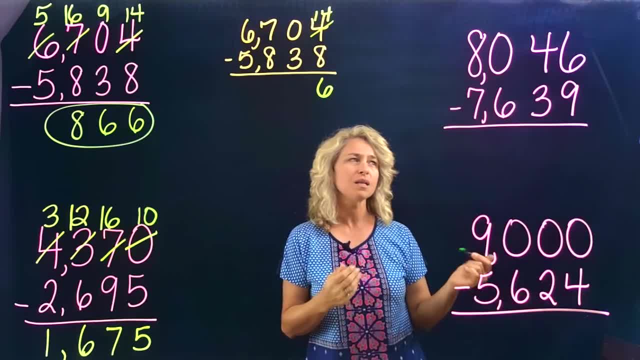 moving the 0 now is in a different spot. moving the 0 now is in a different spot. it can be in any location. let's see what. it can be in any location. let's see what it can be in any location. let's see what. if this is going to be an example of 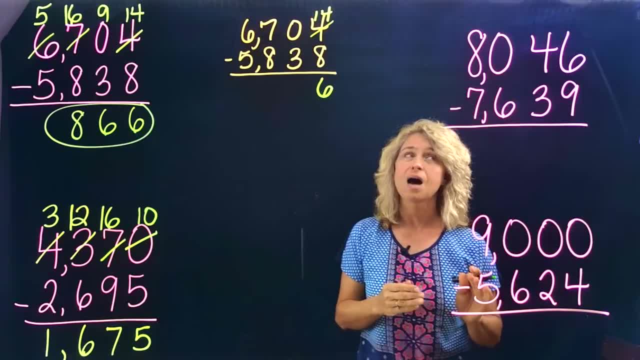 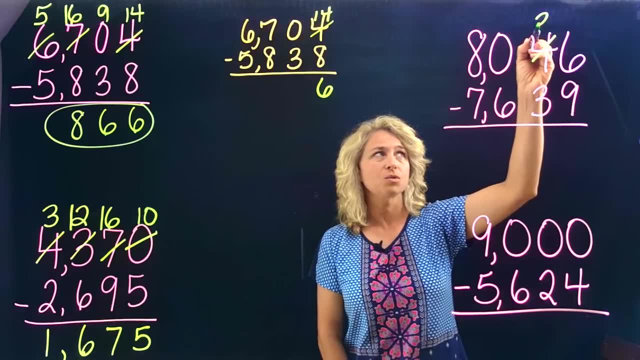 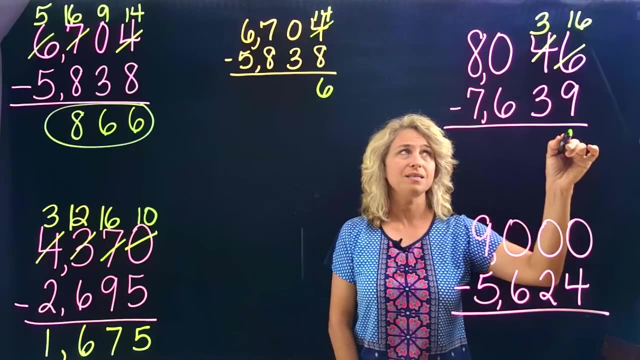 if this is going to be an example of, if this is going to be an example of going across, or, let's see, if it's going to be one where we stop 9 minus 6, take away and borrow from the next door. it becomes one less. now the 6 is 6 plus 10, which is 16. 16 minus 9 is 7. 3 minus 3 is